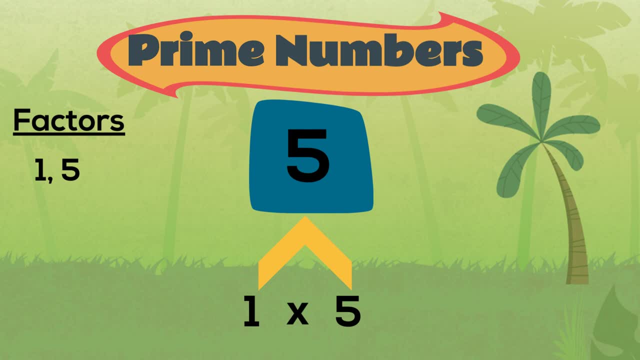 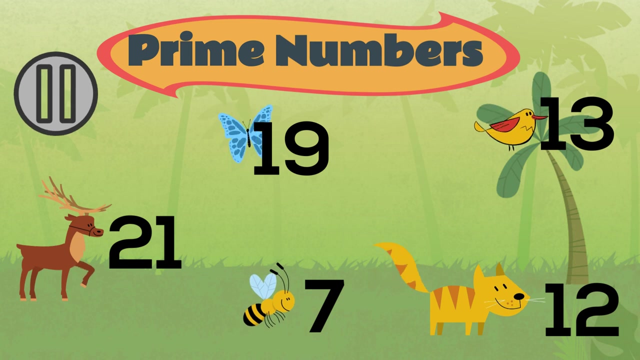 multiplied together to make five. This means that five has two factors: one and itself. Five is a prime number. Look at these numbers and see if you can work out which of them are prime numbers, Which of these numbers have only one and five. 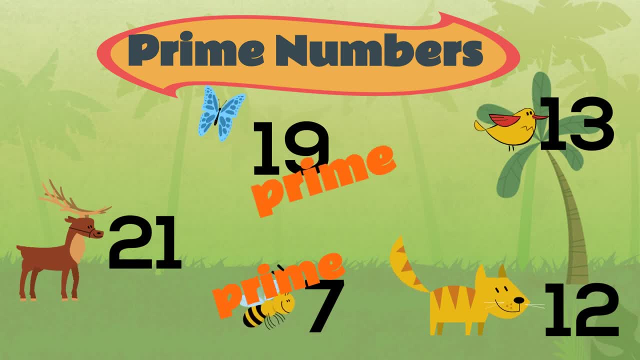 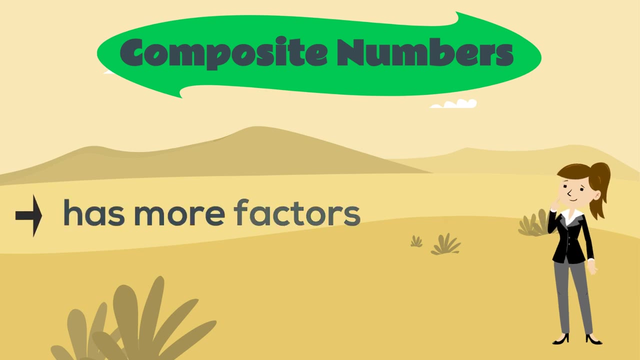 Seven, nineteen and thirteen. Seven, nineteen and thirteen are prime numbers. Now let's look at composite numbers. A composite number is a number that has more factors than just one and itself. Remember, when we looked at the number four, We found out that its factors were one. 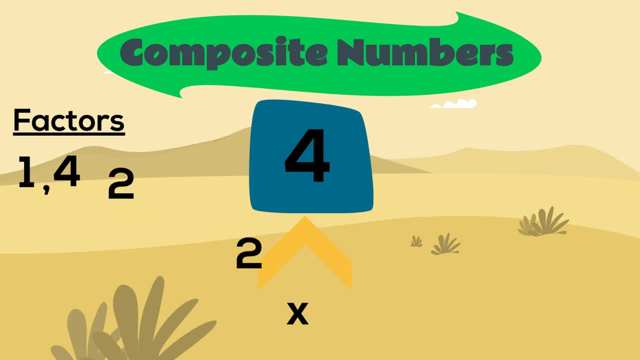 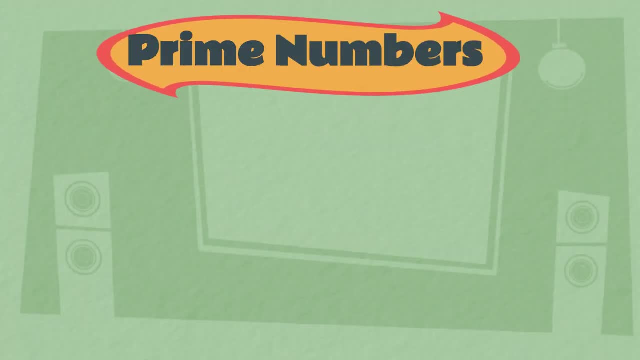 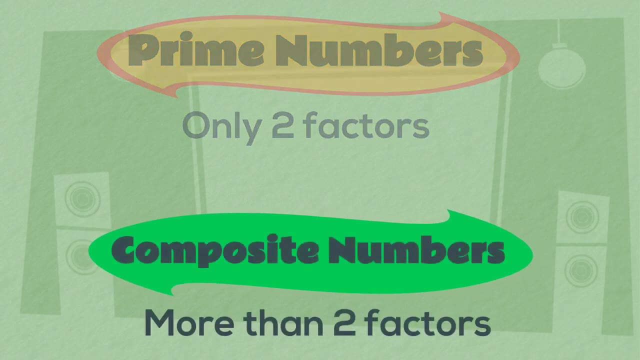 four and also two, Because four has more factors than just one and itself it is a composite number. Prime numbers have only two factors. Composite numbers have more than two factors. A whole number is either prime or composite. It can't be both. 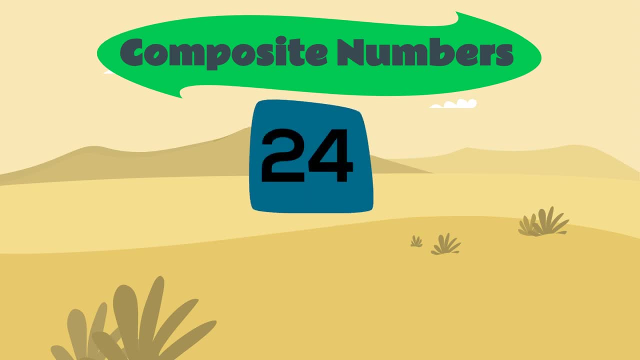 Let's take a look at the number twenty-four. To decide whether it's prime or composite, we'll need to work out its factors. We know that every number has one and itself, so let's start there: One and twenty-four. There is also two and twelve. 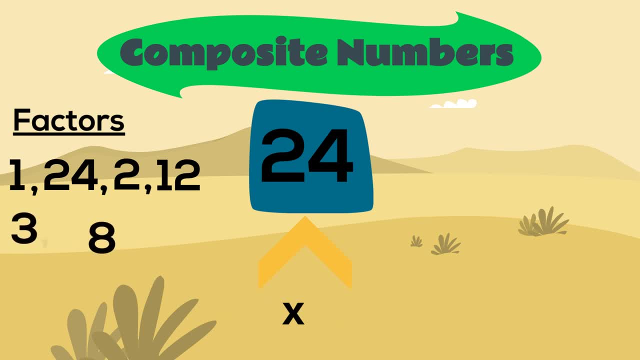 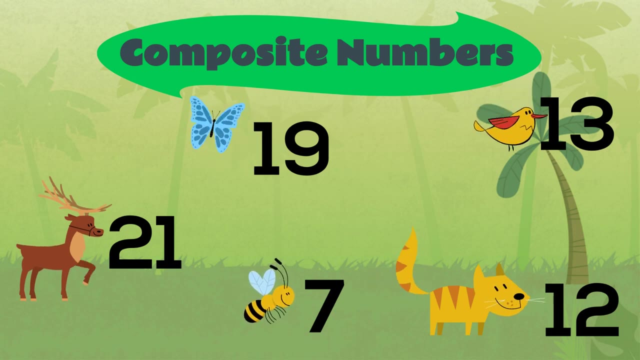 Three and eight And four and six. We know that the number twenty-four has more than two factors, which makes it a composite number. Take another look at these numbers, Which are composite numbers, That's right: Twenty-one and twelve. They each have more factors than one and themselves. 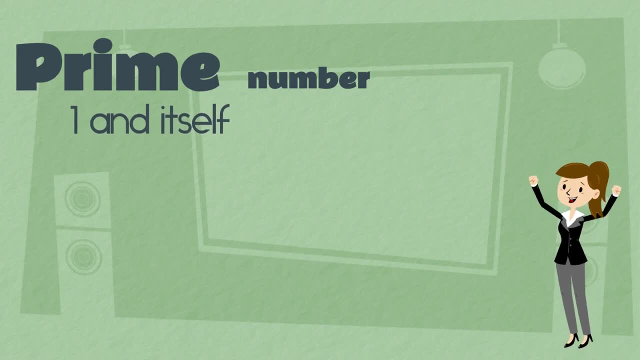 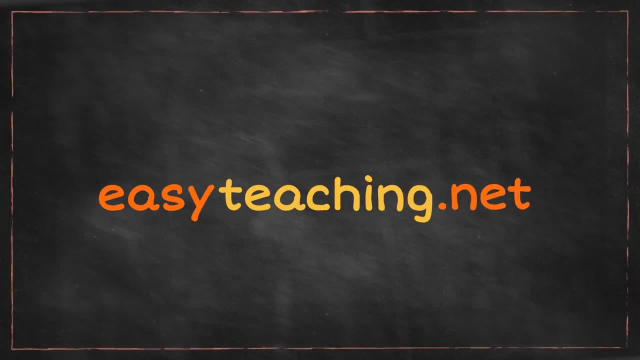 A prime number has only one and itself as factors. Composite numbers have more. EasyTeachingnet- wwweasyteachingnet.